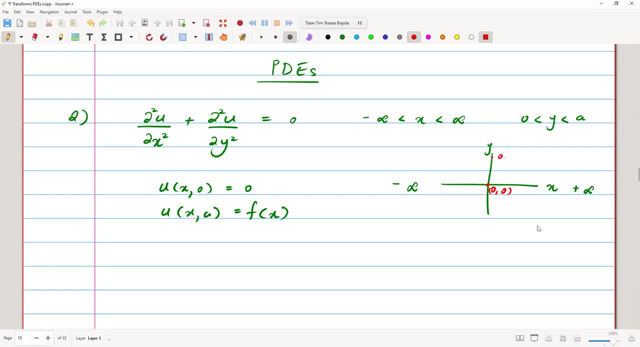 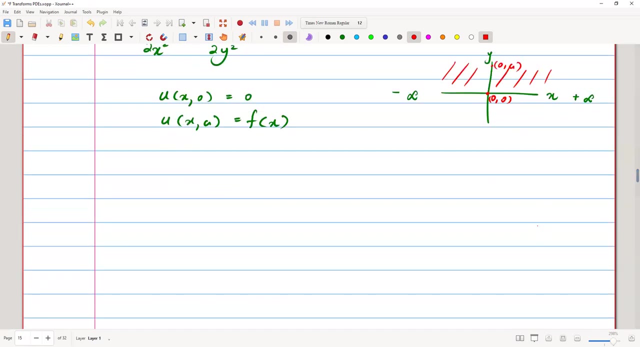 here. that is a zero comma, or you can say zero comma a. Okay, fine, So it's the upper half plane, this whole upper half plane. we are going to compute this Fourier transform of this partial differential equation. So let's apply. 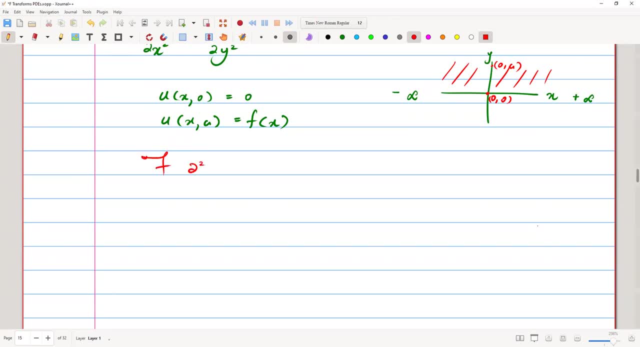 the transformation on the equation And as we know that the boundary conditions are given for y, So we are going to apply the transformation in that appropriate manner. So transformation we applied, And then what we will get here. so we know that x is from negative infinity to positive infinity. So this is the 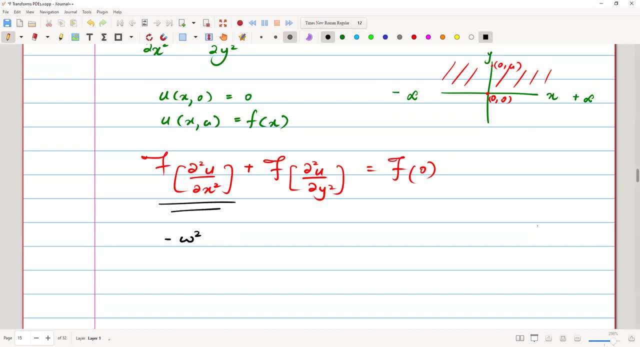 subject of transformation. we are applying transformation with respect to x, So it's negative omega squared u, and then plus it will be d. d squared. u over d. y squared equals zero. Okay, so now we have a second order, homogeneous differential equation with constant coefficients, And we know that. 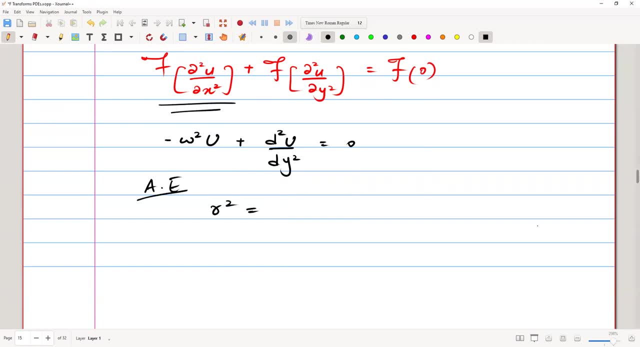 we can solve it by using the auxiliary equation. So it's: R squared equals Omega squared, which implies R equals plus minus Omega. So the solution can be written as: a? e to the power omega y plus b? e to the power negative omega y. 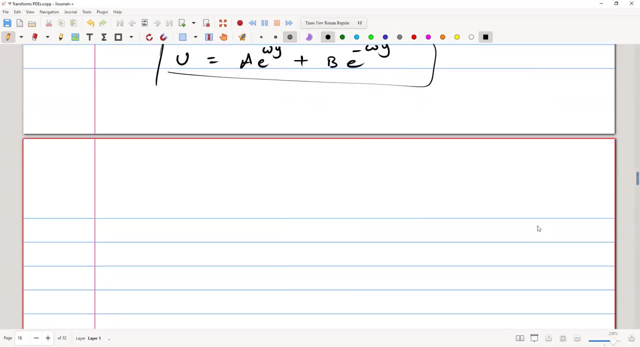 So this function, what we get is a function of omega and y, but we need a function in terms of x and y. So therefore, first of all, we need to apply the boundary conditions. So, before applying the boundary conditions, we have to take the transformation of the boundary conditions. 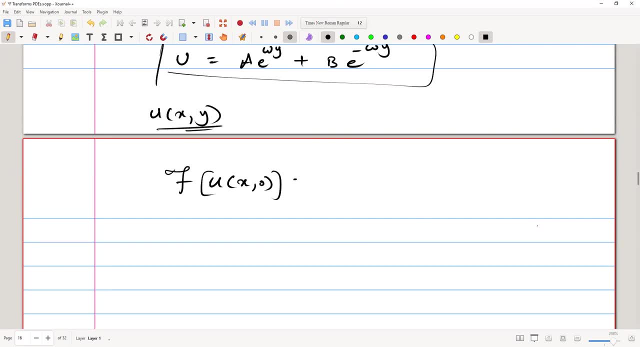 So the Fourier transform of this boundary condition is going to be Fourier applied on the boundary, So it's zero. Therefore u omega zero is again zero. And for the second condition we have u, x comma. a equals some function of x, which means that Fourier transformation. 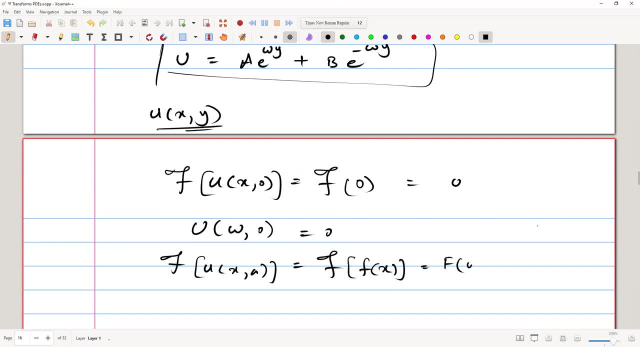 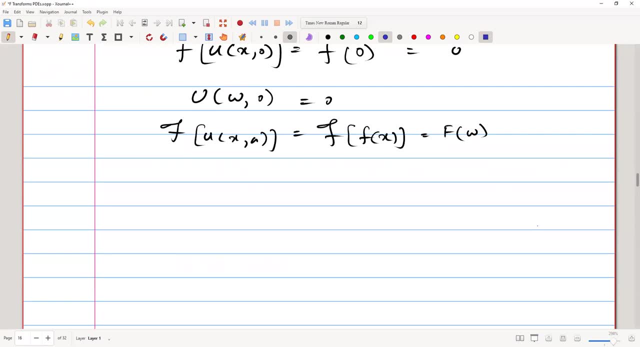 And of some function of x. we all know it's again a function of omega. So we can write like this: Then what we need to do is we need to apply the boundary conditions, So u of omega comma zero. it simply means that a to the power zero plus b, e to the power zero, equals zero. 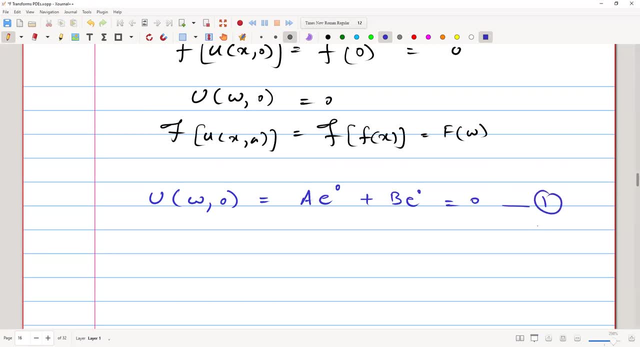 This is equation number one. And then we have u of omega, comma a. That is equals two A, e to the power, negative omega a plus b e to the power. omega a equals f of omega. All right, So from this equation that is, 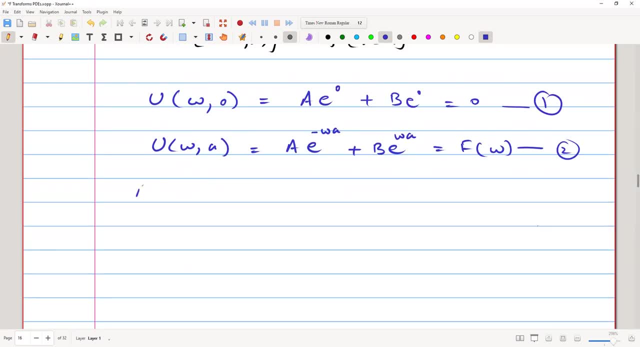 So let's call it equation two. So from equation one it implies that a is equals to negative times b. So we can just plug it in equation two. So you get negative b e to the power, negative omega A plus b e to the power. omega a equals function of omega. 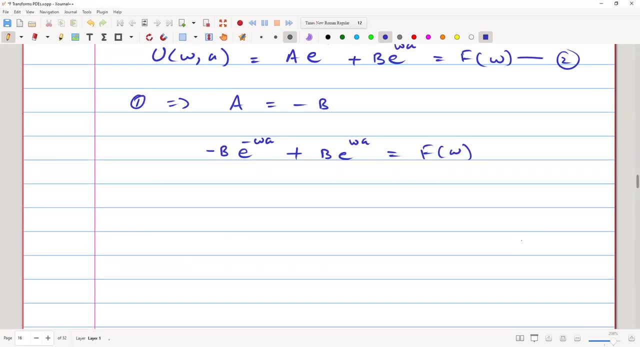 So from here we can use the identity, So we can take out b as common. In fact we'll take negative b as common or take it positive b as common, So we'll get e to the power omega a minus e to the power negative omega a. 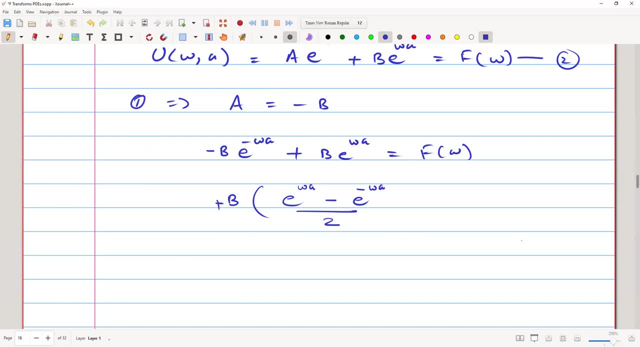 And if you divide it we'll get negative b. So we have to multiply it by two. So we have to multiply here by two as well. Therefore, we are going to get a hyperbolic function. We know that right. 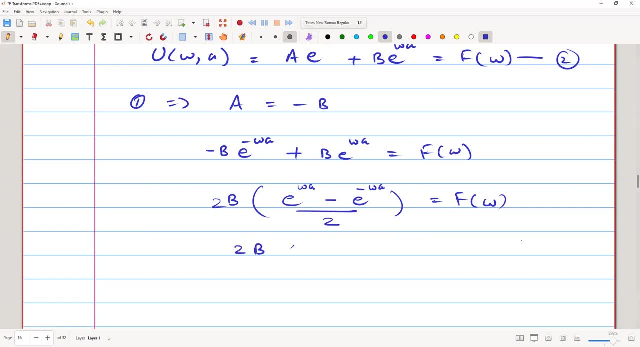 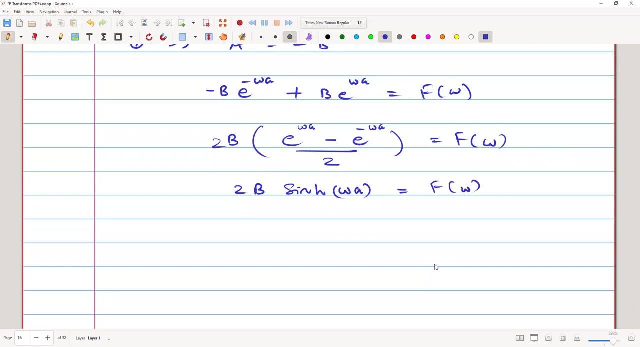 So two b sine hyperbolic omega a equals f of omega. All right, Now we have this hyperbolic function here, So we can take out b? e to the power negative omega a, plus b e to the power negative omega a, so we can write: b of omega is nothing, but it's equals to f of omega divided by two times sine. 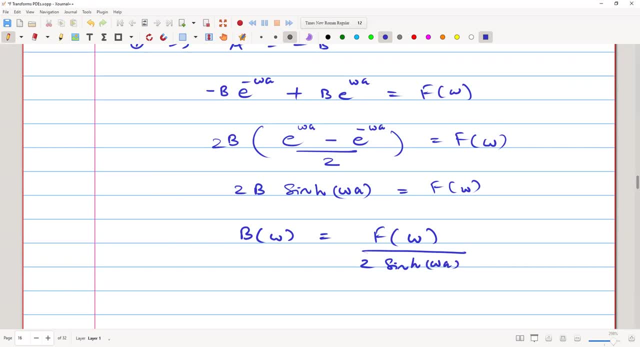 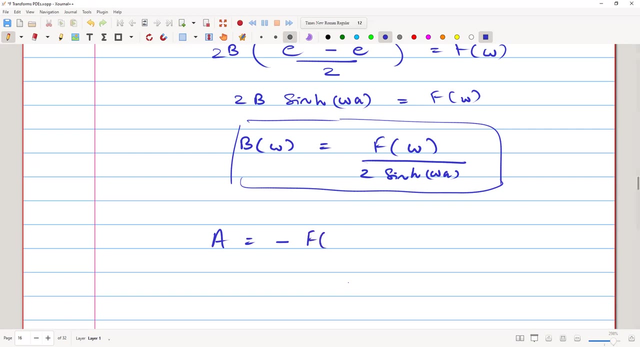 hyperbolic omega a. okay, now we know that b is uh, a is equals to negative times b, so we can write: a equals to negative times, this whole expression. so it's negative times for f of omega divided by two sine hyperbolic omega a, and then we can plug this in the equation of u omega. 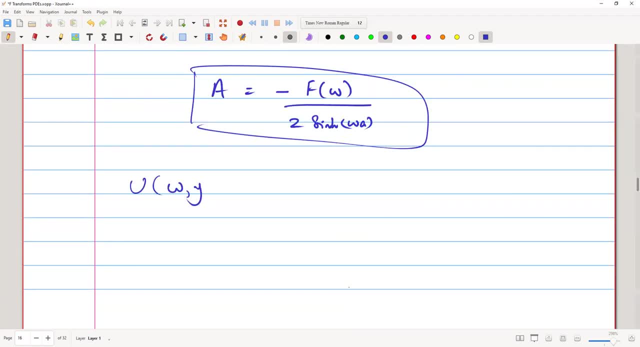 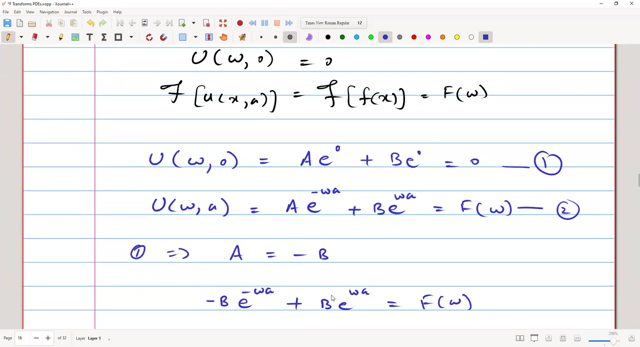 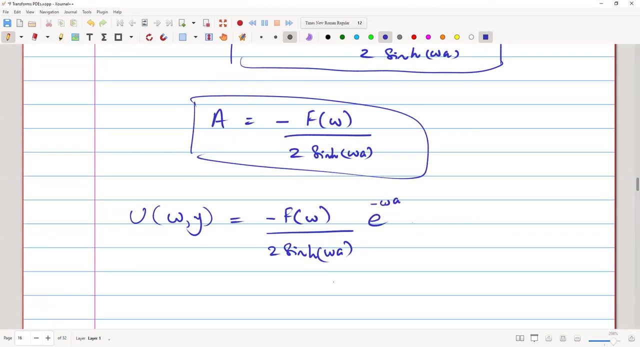 y, so it's u. omega y is now equals to negative f of omega divided by two. sine hyperbolic omega a times e to the power. we have negative omega a, so it's negative omega a plus f of omega divided by 2. sine hyperbolic omega a times e to the power. 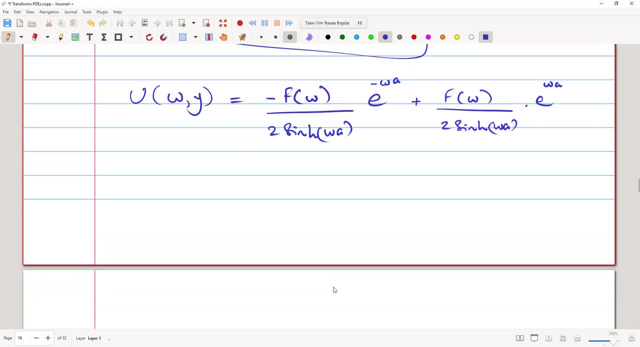 omega a right. so now this is the expression uh for u omega y, but we need in terms of uxy. so what we can do is we can take the inverse transformation and again we have this function common here, this and this, so we can take it out common. 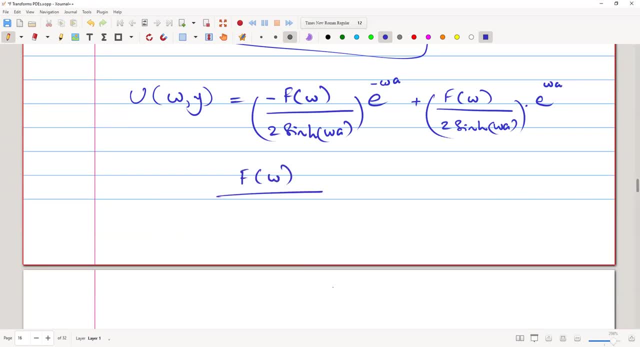 so we will get f of omega divided by two sine: hyperbolic: omega a. times heel power: omega a minus yield power negative omega a. okay, oh, uh, one thing i just missed. here is omega y, not omega a. sorry for that. uh, because we have function of omega y now. okay, so this is omega y. and again, if we divide it by two, 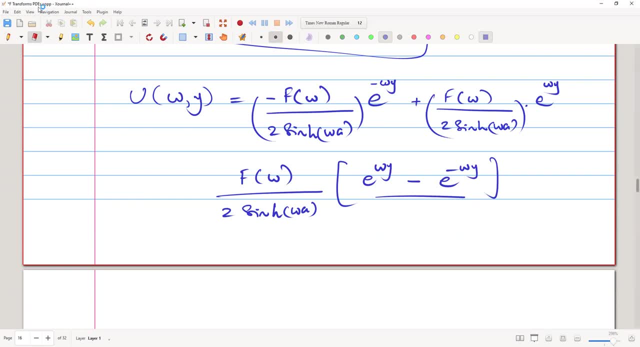 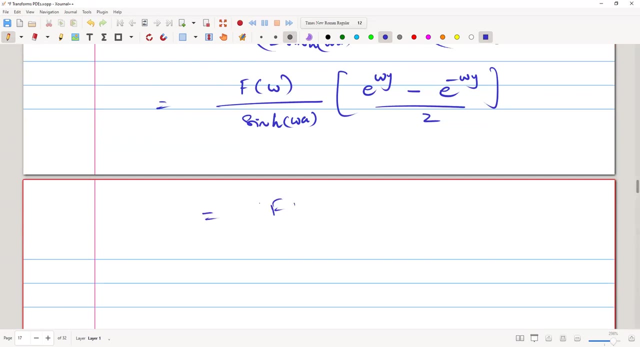 we don't need to actually to divide it by two, because we have two here. so this two we can simply move inside. so let's do it here just right to here. and then we have f of omega times, sine hyperbolic omega y again, and then divided by sine hyperbolic omega a. now, this is the.